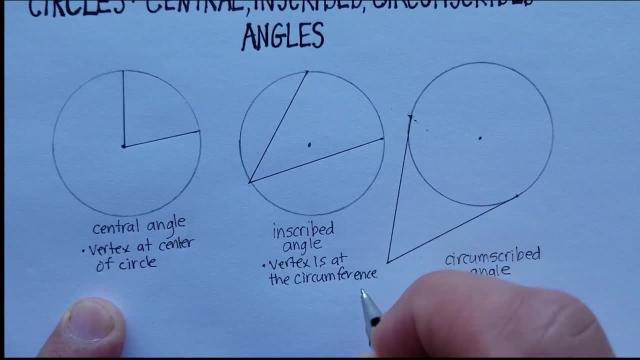 or the perimeter, Although we usually use perimeters for, like, hard-sided figures. we call it a circumference. So the vertex is at the circumference and for a circumscribed angle, the vertex is located outside the circle. So out here, okay: vertex outside circle. 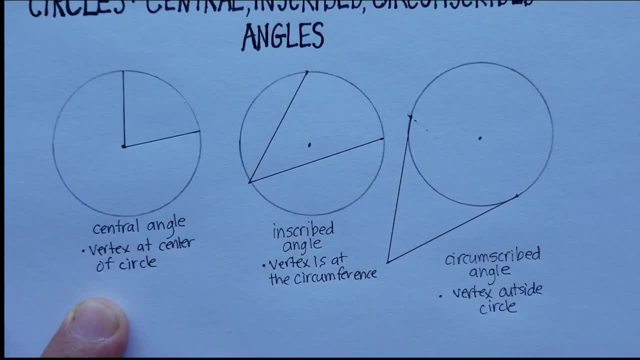 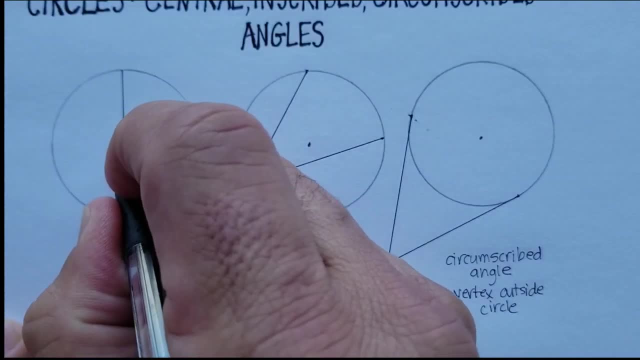 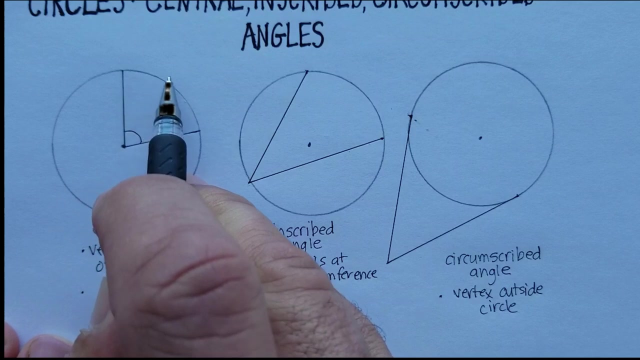 And because of that they each have different kind of characteristics on how you would calculate them. So, for example, in a central angle like right here, the number of degrees here it'd be equal to the number of degrees of the arc. Okay, so the angle. 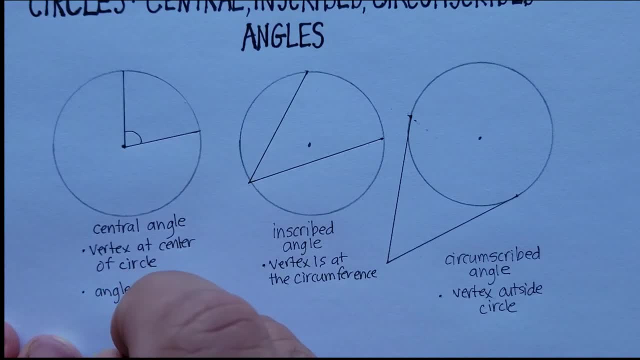 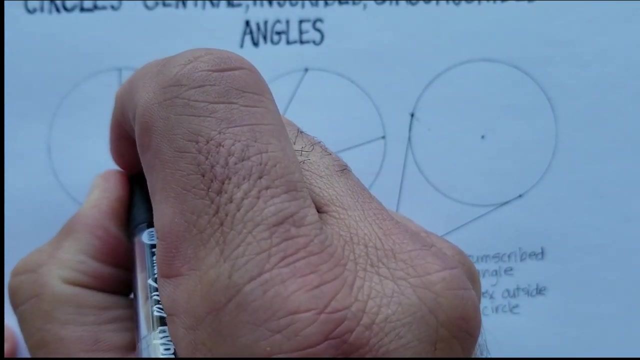 is equal to the what they call an intercepted arc. Okay, and that's just for a central angle only. So if this were, let's say, 80 degrees, then this would be 80 degrees as an example. Okay, So if that were? 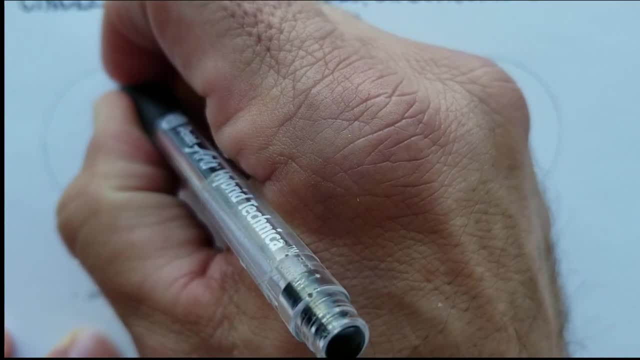 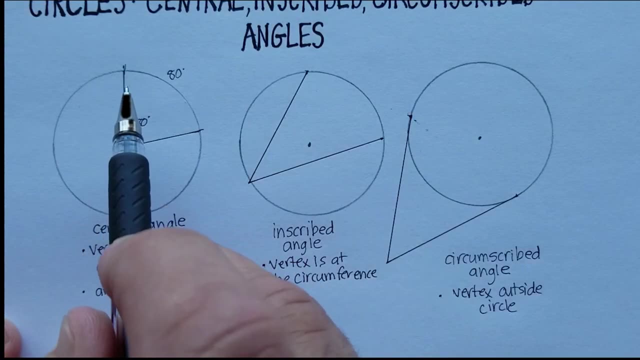 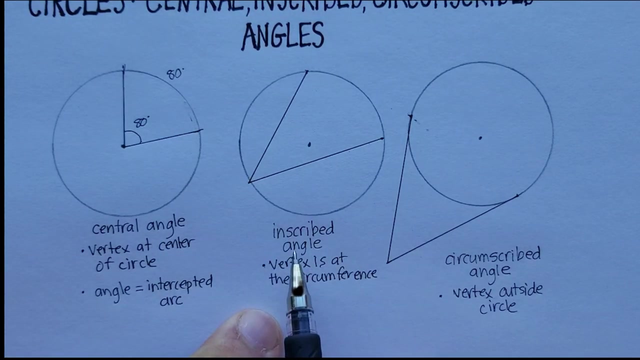 80 degrees. that means that the arc is also 80 degrees. All right, And remember, the arc is that portion of the outside. Sorry about that. The arc is that portion of the outside of the circle. Okay, Now for an inscribed angle. it's a little bit different. The angle itself is one half. 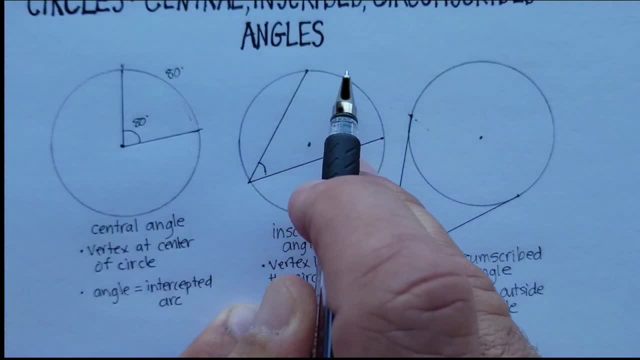 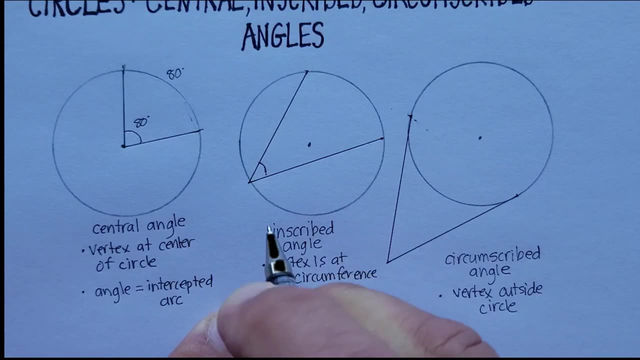 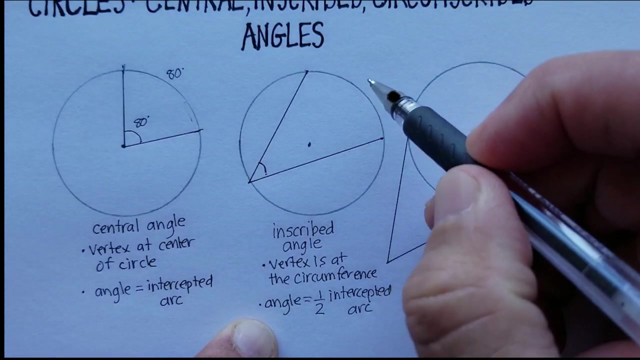 the number or one half, the measure of the intercepted arc. Okay, So the angle of an intercepted inscribed angle is equal to one half intercepted arc. Okay, So if, for example, again let's say that the arc were 80 degrees, 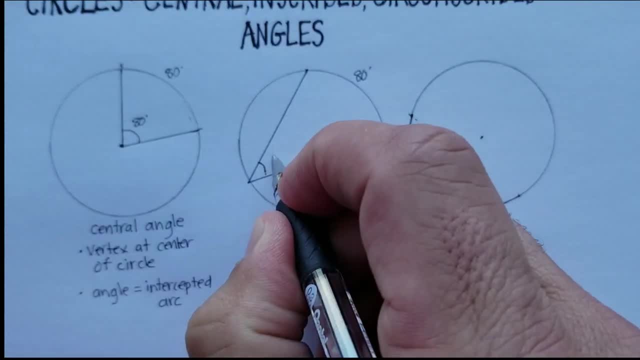 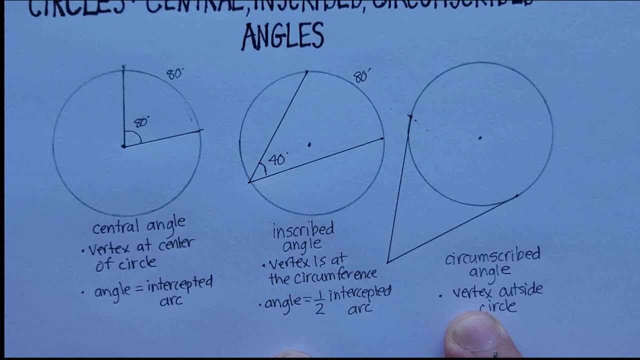 that means that the angle would be 40 degrees. Okay, You can always count on that. Now for a circumscribed angle. it's going to be a little bit more complicated. Let me describe what happens here. A circumscribed angle has two. 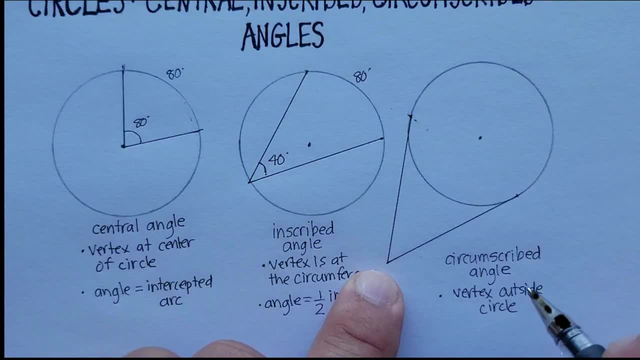 rays All right That are tangent to the circle. So let's just let's do that first: Two rays tangent to the circle. Now it doesn't have to be just a ray, It could also be just a line, like this one, For example: 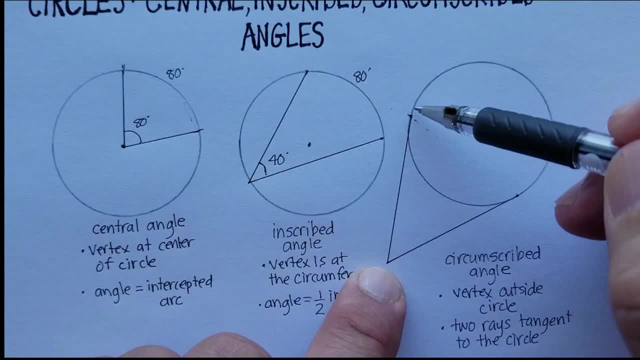 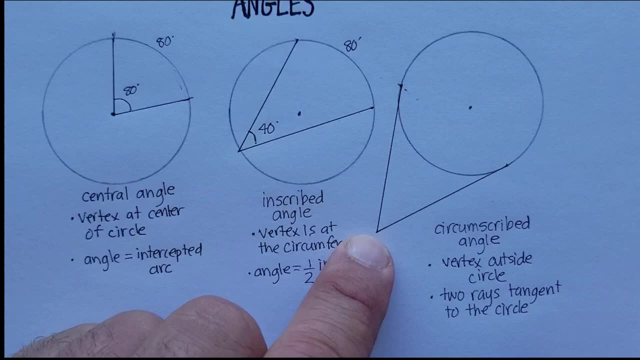 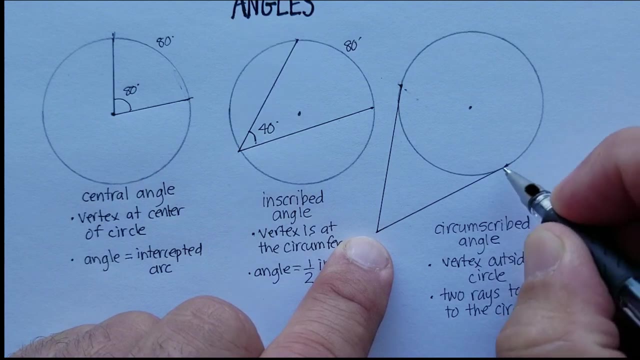 it ends right there, or a line segment, or a line segment, But for a ray, remember, we just continue on In both directions. But the point is that a tangent line intercepts the circumference at only one spot. All right, So there is just one point that intersects the circle. 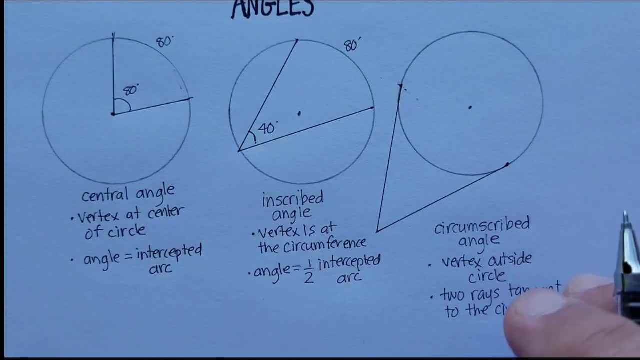 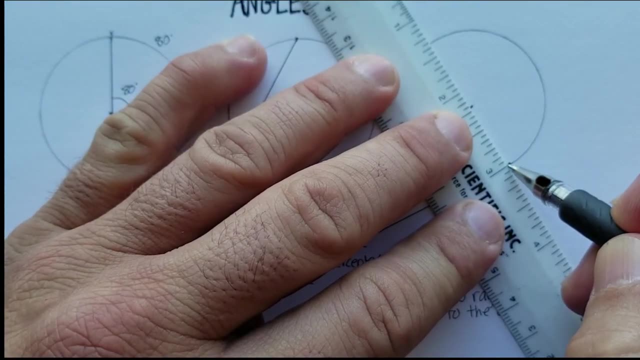 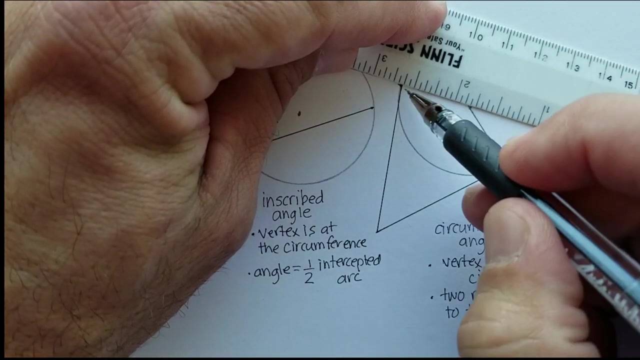 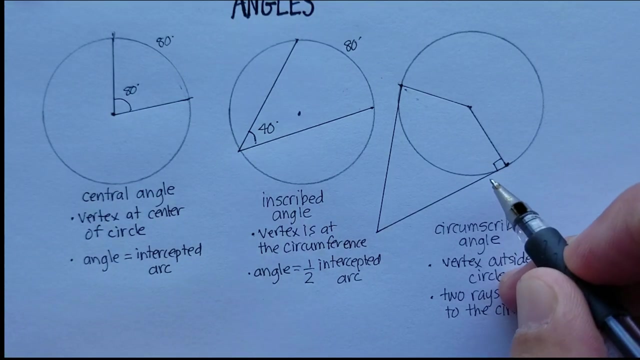 So that's what a tangent line does. The cool thing about tangent lines is that if you were to draw a line from where it intercepted to the center of the circle, like that, and another one like that, Let's do that. The angle that it forms is always 90 degrees. 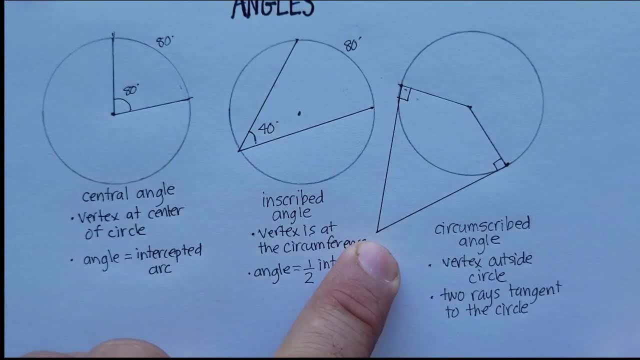 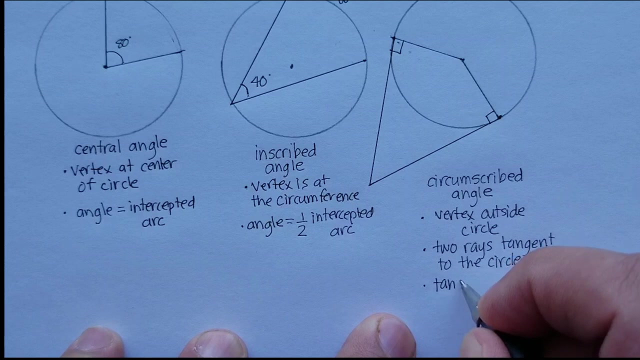 Okay. The angle that it forms is always 90 degrees, So tangent lines create 90 degree angles with the center of the circle. Let me write that down, because that's really an important thing to do. Tangent lines, Tangent lines. 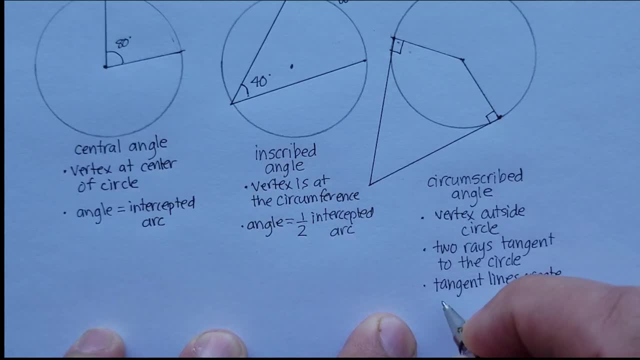 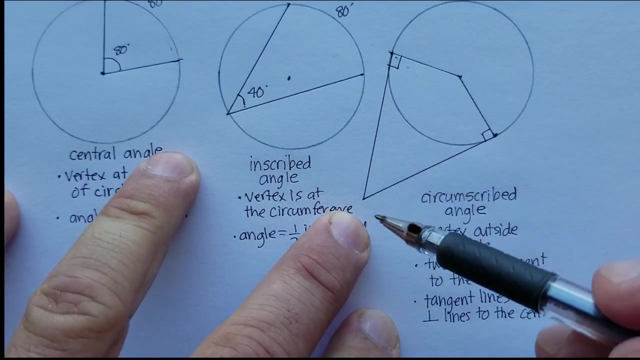 Create perpendicular. This is a symbol for perpendicular, Remember perpendicular angles or perpendicular lines to the center of the circle. Okay, But it also does something else. This circumscribed angle notice is a four-sided figure. Now this particular figure is called a kite. 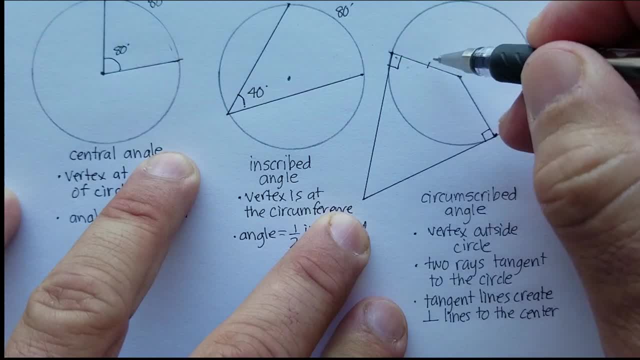 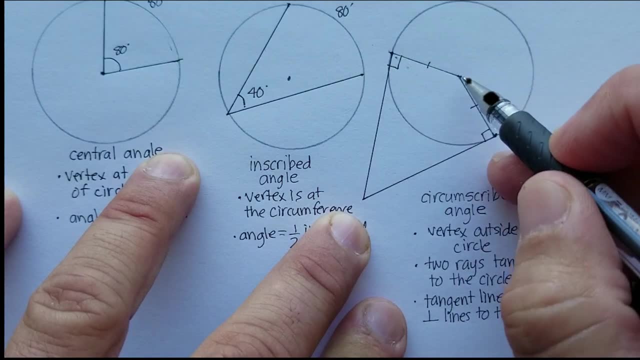 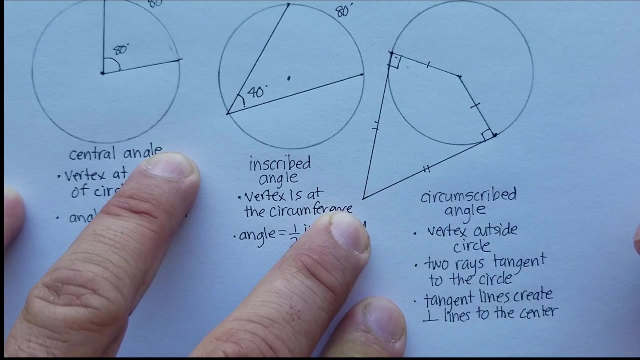 Remember what a kite is. That means that there are two consecutive congruent lines, So this segment, this line and this line are congruent, And then this line and then the consecutive line after it is also congruent. That's kind of important because in a kite 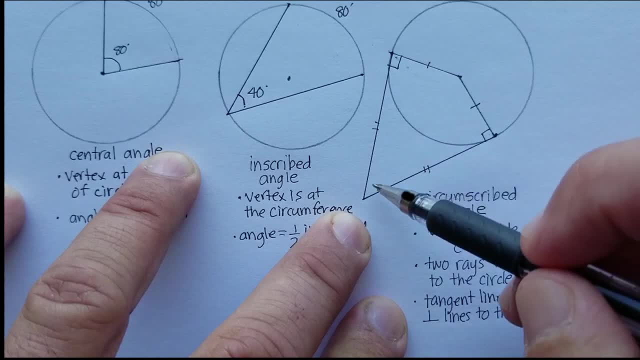 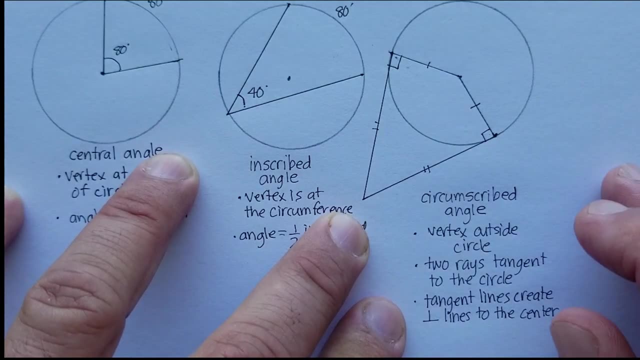 the opposite sides of a kite are always supplementary. Let me say that again, because that's again a little bit more complicated. I told you that this part is going to be a little bit more involved, All right, So let's say that again. 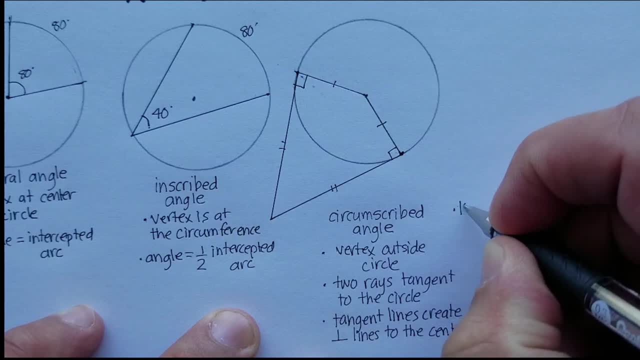 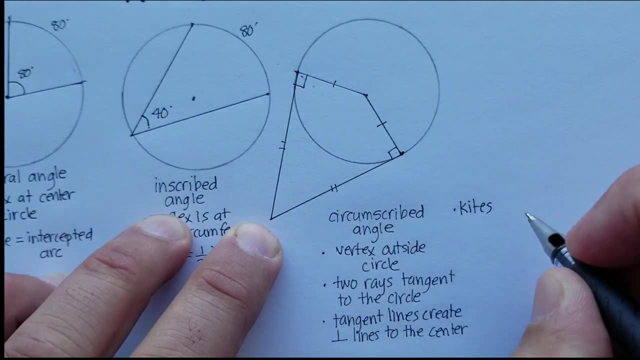 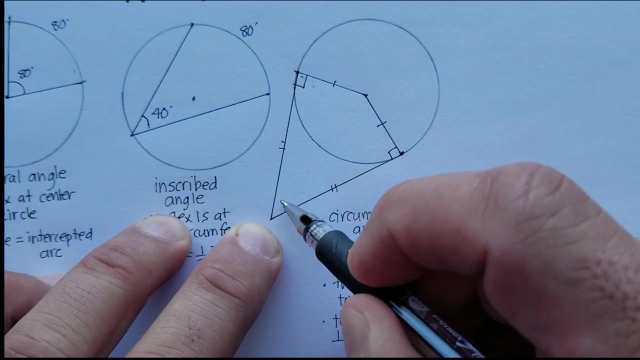 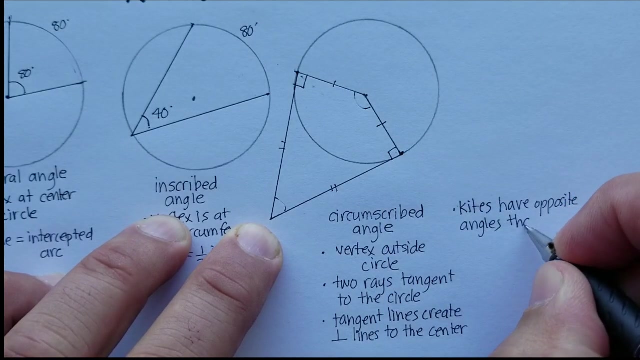 So kites will always be formed by these tangent lines. right Kites have opposite sides, Opposite angles. So this one and this one, for example, and this one and this one, that are complementary- Excuse me, that are supplementary. 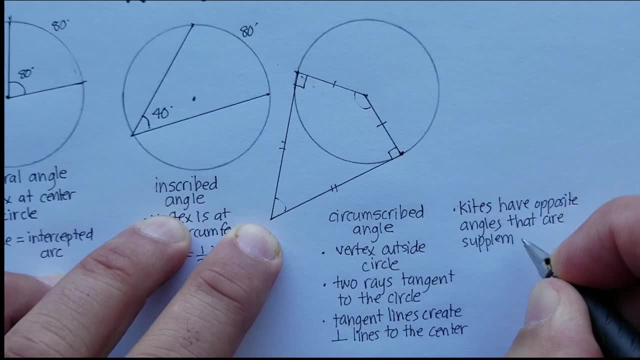 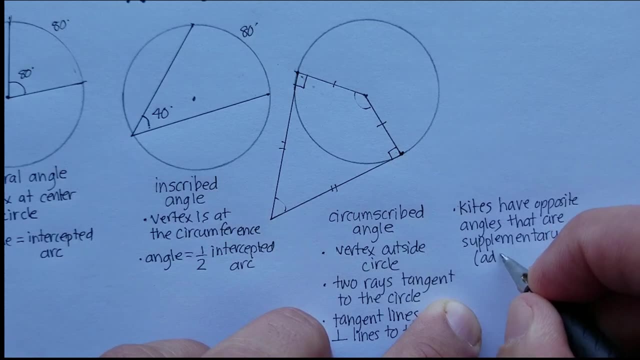 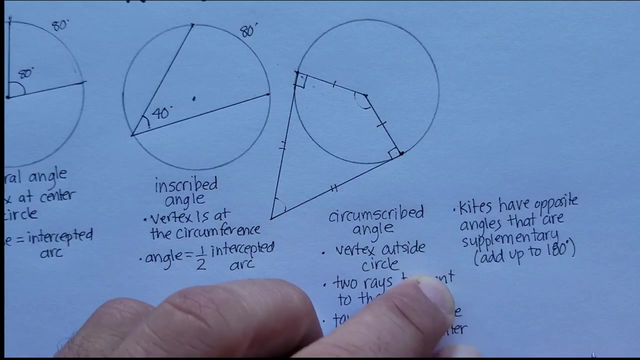 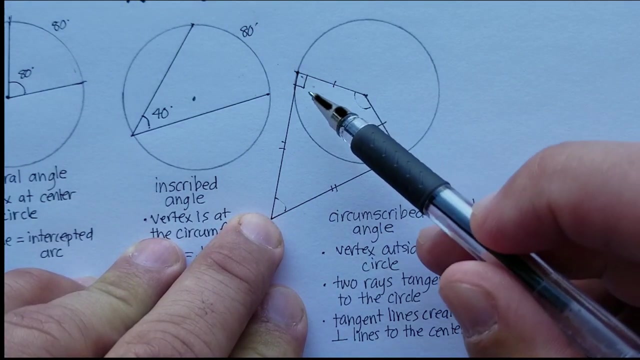 And remember that supplementary means 180.. They add up to 180 degrees. Now that makes some sense with our perpendicular lines, doesn't it? Our perpendicular angles, Since these are opposite each other and we know that they are tangent lines, we know they form right angles. 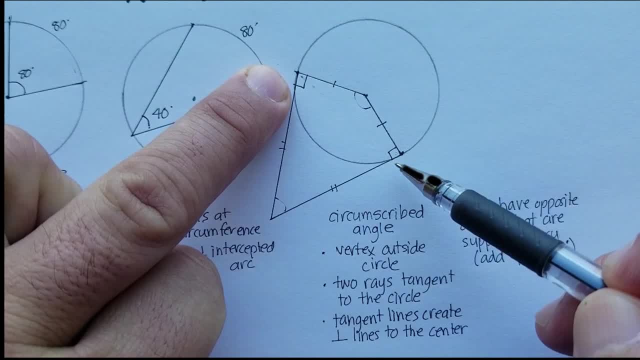 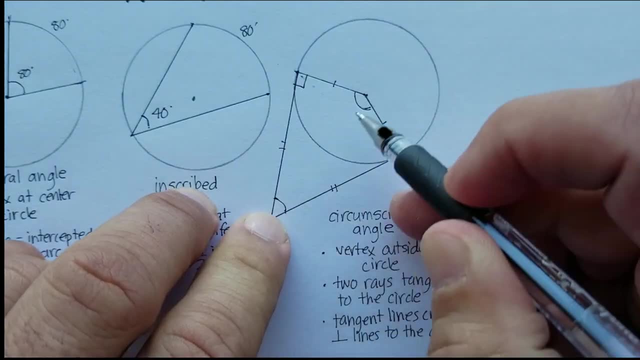 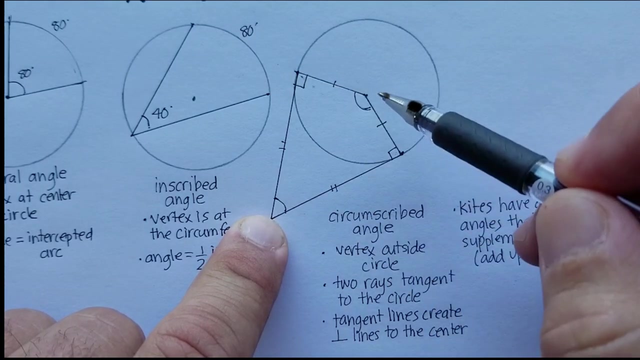 This angle and this angle add up to 180 degrees, which means that this angle and this angle, this angle and this angle must add up to 180 degrees. Now, why do we know that? We know that because in a quadrilateral, four-sided figure, 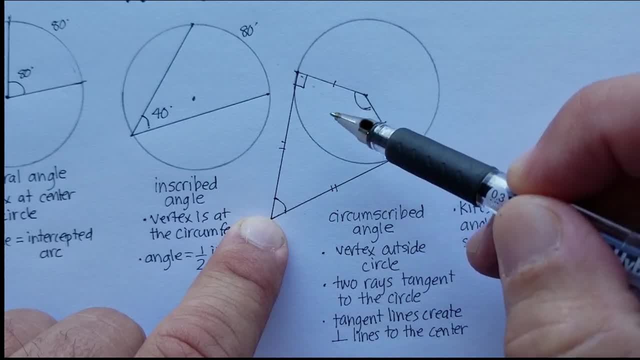 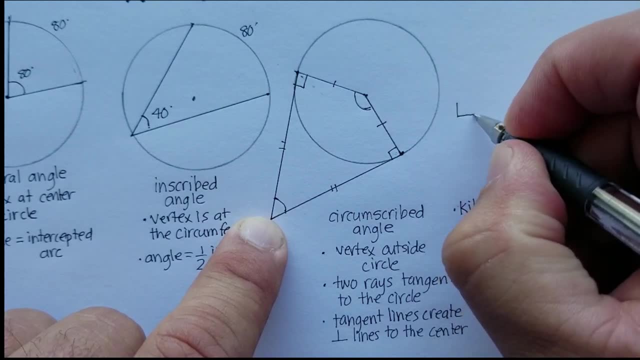 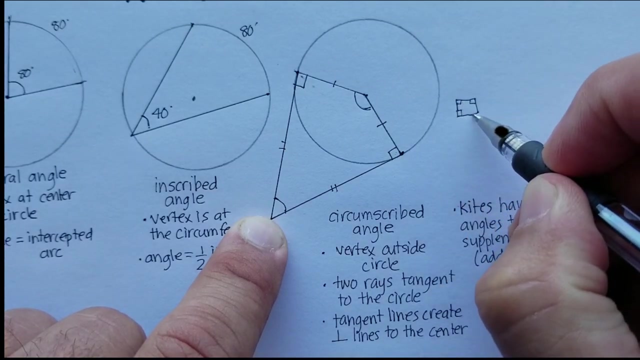 there are 360 degrees that make up the internal angle of a four-sided figure. Remember that If you want to have proof of that, just remember that a box or a square, if you add all those, a four-sided figure has four 90-degree angles. 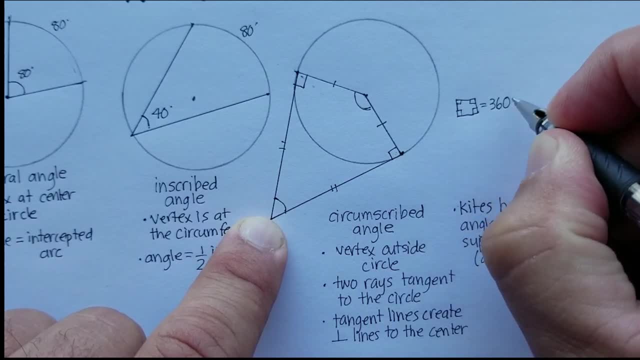 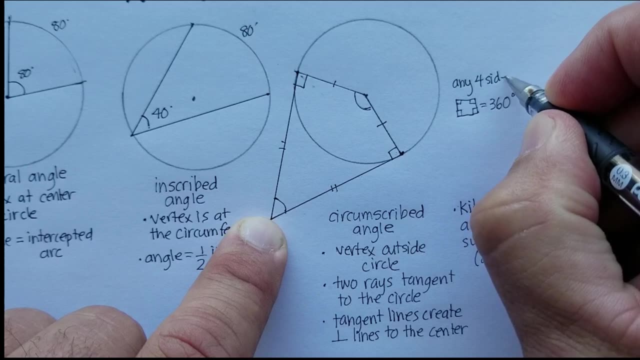 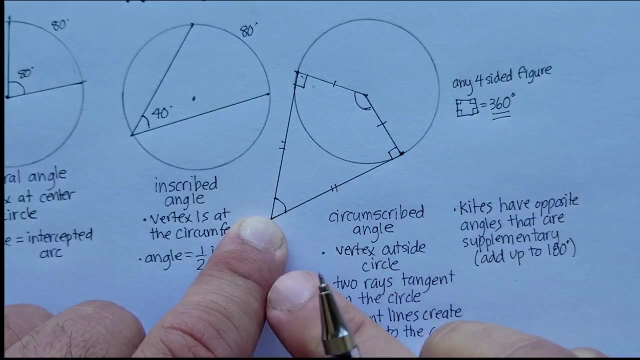 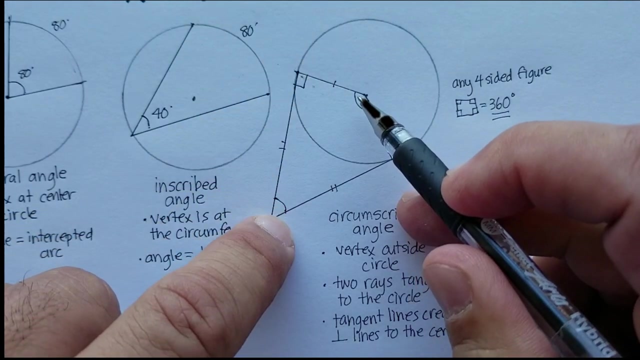 Those equal 360 degrees. In fact, any four-sided figure has internal angles that equal 360.. In this kite, no matter how stretched out it might be, the opposite sides always equal 180.. That's actually pretty helpful, Okay, Because if, for example,